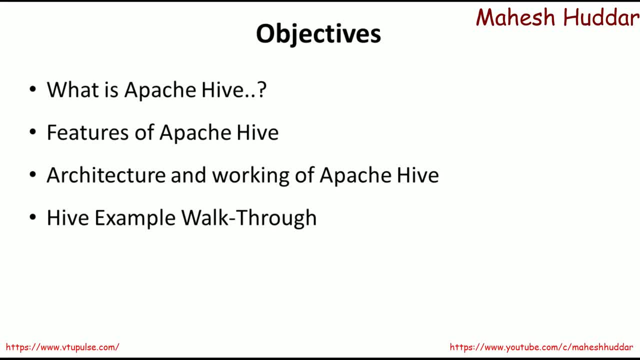 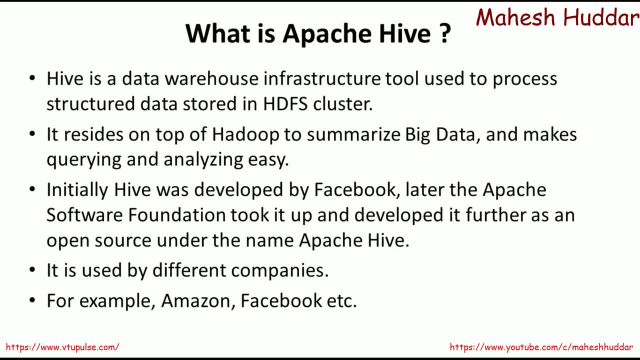 understand HiveQL query language. What is Apache Hive? Hive is a data warehouse infrastructure tool used to process structured data stored in HDFS cluster. Hive resides on the top of Hadoop to summarize big data and makes querying and analyzing data very easy. Initially, Hive was developed by Facebook. Later, 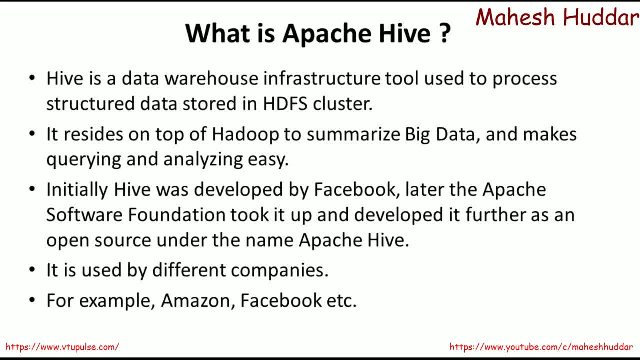 the Apache Hive was developed by Hadoop. Later the Apache Hive was developed by Hadoop. Later the Apache Hive was developed by Facebook. Later the Apache Hive was developed by Facebook. Software Foundation took it up and developed it further as an open source under the name of. 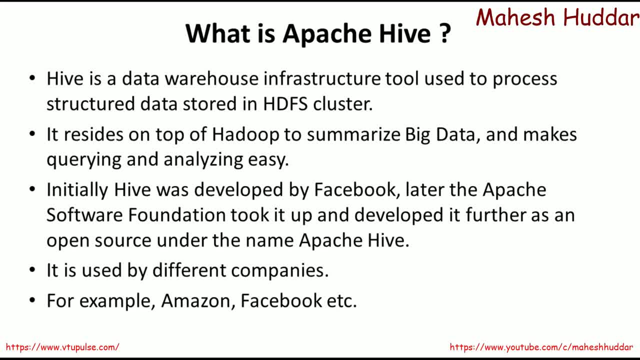 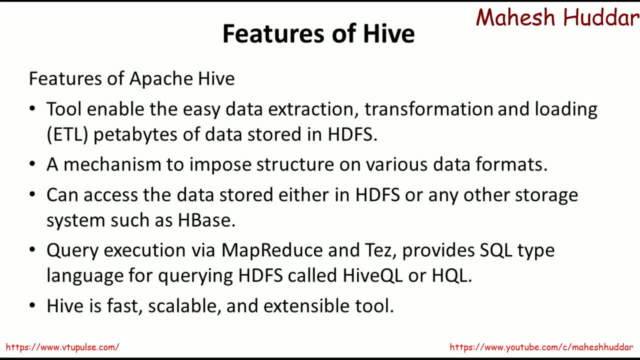 Apache Hive. It is used by various companies such as Amazon and Facebook, etc. What are the features of Apache Hive? If one wants to extract, store, transform and load a petabyte of information which is stored in HDFS, he can use Apache Hive tool. 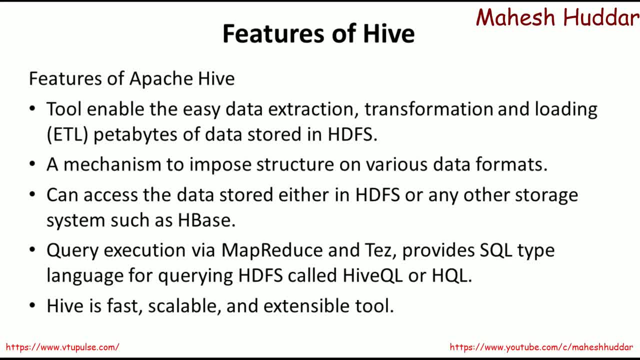 Apache Hive tool imposes structure on various data Formats. One can access data stored in HDFS or other storage systems like HBase. Apache Hive allies. SQL-type language called HiveQL habla will query theWhite and whiteій Horizon data which is stored on hdfsChromaSceptaCul. 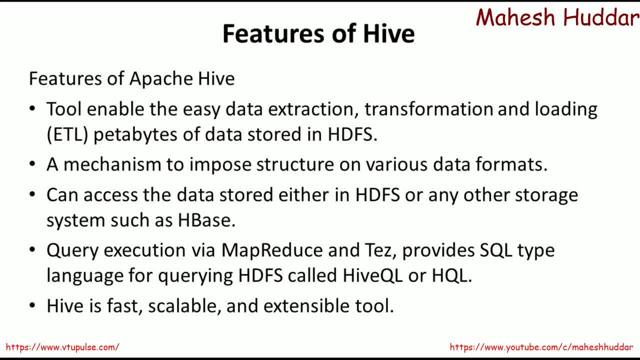 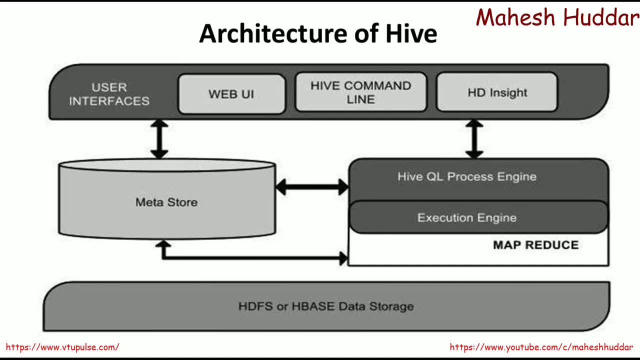 ApacheHive provides SQL-type language called HiveQL or hql to query the data which is stored on HDFScluster. Hive is fast, scalable and extensible tool. Now we will see what is the architecture of Apache Hive. Apache Hive has five components. 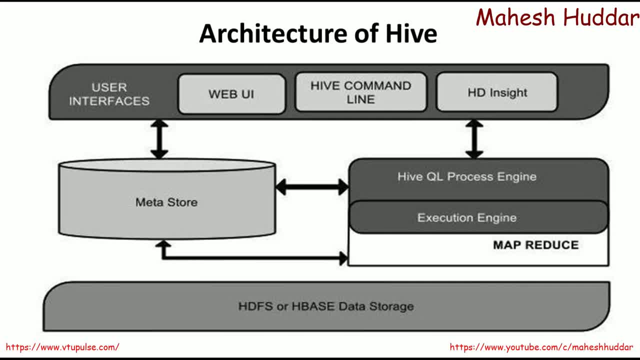 The first component is user interface, second one is metastore, third one is HiveQL process engine, fourth one is execution engine and fifth one is HDFS or HBase data storage. Hive provides three kinds of user interfaces. One is the web UI. here the user can access the Hive UI Hive tool with the help of browser. 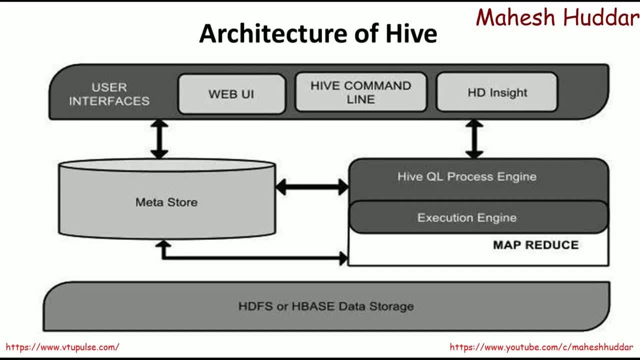 The other way to access Hive tool is with the help of command line, where the user can write a command like HiveQL. HiveQL command can be written on a command prompt so that he can access the Hive tool. The third one is an application called as HDinsight, through which also the user can 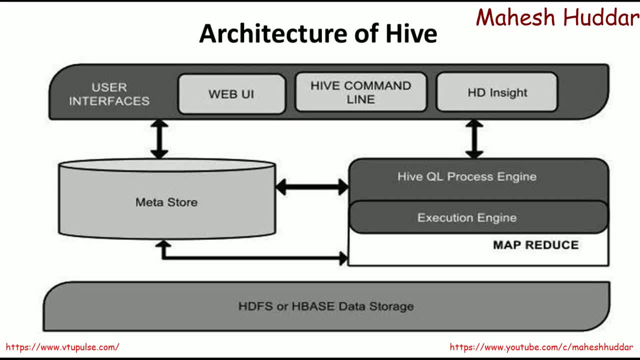 access the Hive tool. The second component is the metastore. Here the metadata information related to database is stored like: what is the database name, what is the schema name, what is the table name, how many number of columns are there in the table, what is the data type of that particular column, and so on. 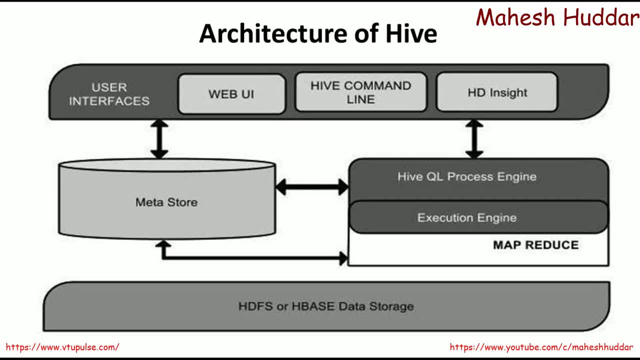 Such kind of information is stored. HiveQL process engine is the component used to process HiveQL queries. Now if user has written HiveQL queries and he wants to execute those particular queries on HDFS cluster directly, it is not possible. So HDFS understands only MapReduce programs. 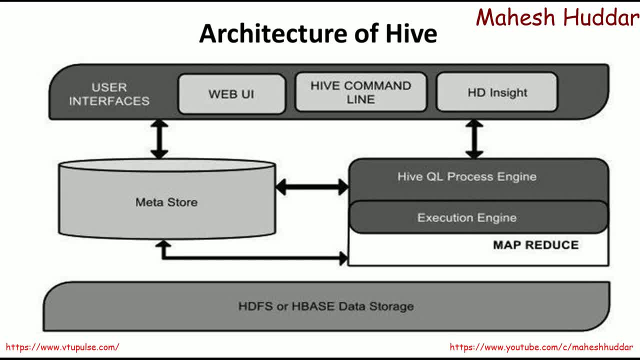 So what is needed is HiveQL queries should be converted into MapReduce programs And then the MapReduce program can be executed on HDFS. So there comes execution engine. What execution engine does is the HiveQL queries written by user will be converted. 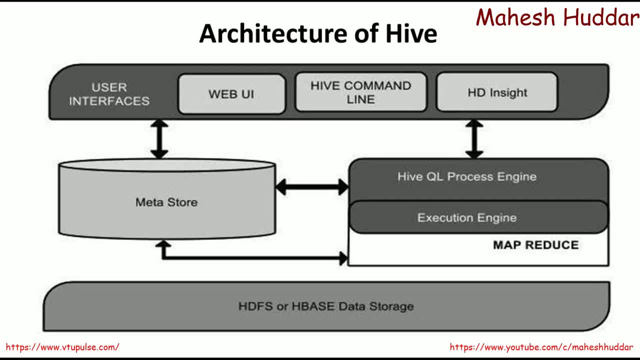 into MapReduce programs and then they will be executed on HDFS or HBase data storage. Once the data is available, the data will be given back to HiveQL by converting the result in the form of HiveQL results. The same results will be given back to the user through user interface. 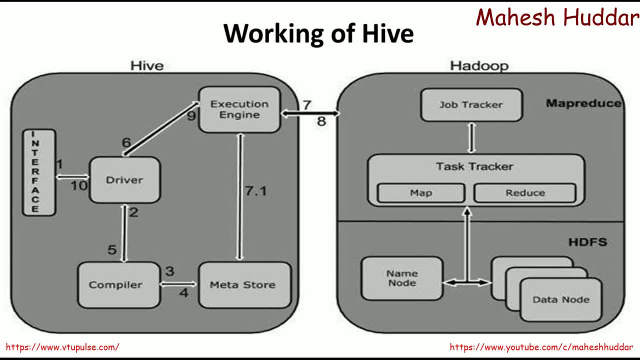 Now we will see how the Hive works. The first user writes the HiveQL queries with the help of either web UI or the command line. Once the user has written the queries, they will be given to the driver. What driver does is: the driver may be JDBC or ODBC. it will send that particular queries. 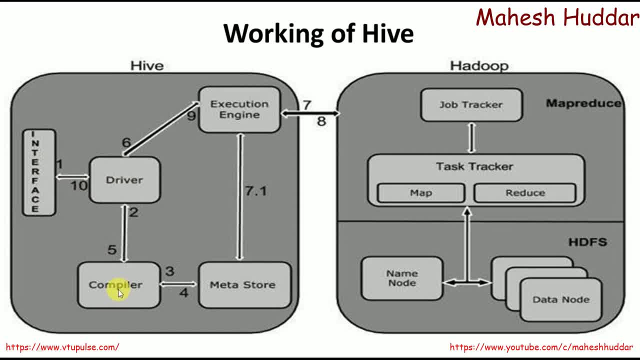 to compiler to check the syntax of that particular query. If the query is syntactically correct, Then the compiler in turn asks the metastore to get the database name, table name, and then the column name, the type of column, and so on. 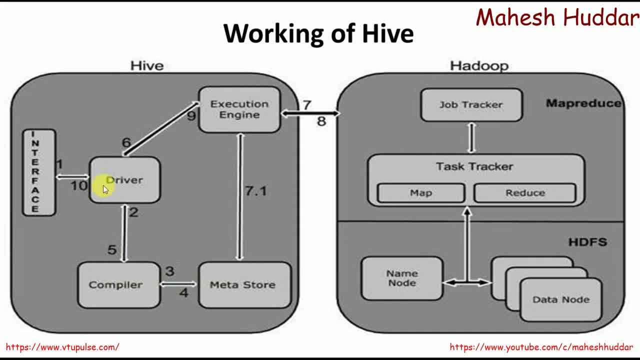 If everything is fine, the compiler sends that particular query back to driver saying that everything is fine with the query. you can start executing the query Now. the query will be sent to execution engine. What execution engine does is before it sends that particular query to Hadoop environment. 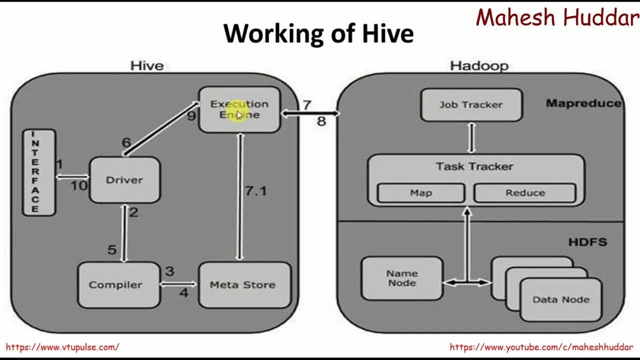 first it gets the metadata information Once again to check the query whether it is correct or wrong. If it is correct, what it does is it will convert that particular query into a MapReduce program with the help of execution engine, and then that job will be executed on that. 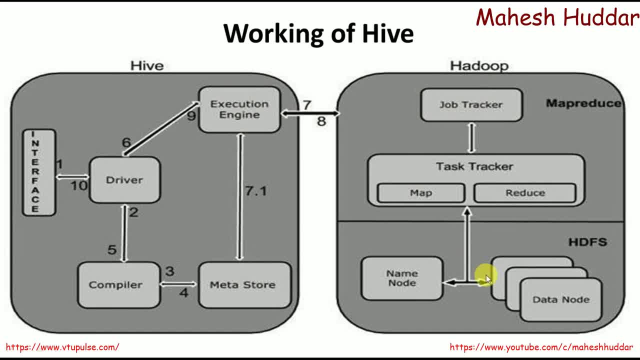 is MapReduce job will be executed on Hadoop environment and then it will get the data from HDFS cluster. Once the data is available, or the result is available, it will be given back to execution engine. The execution engine converts that particular data into in the form of HiveQL result and 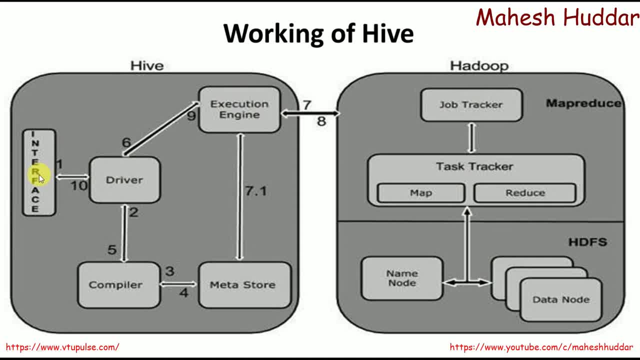 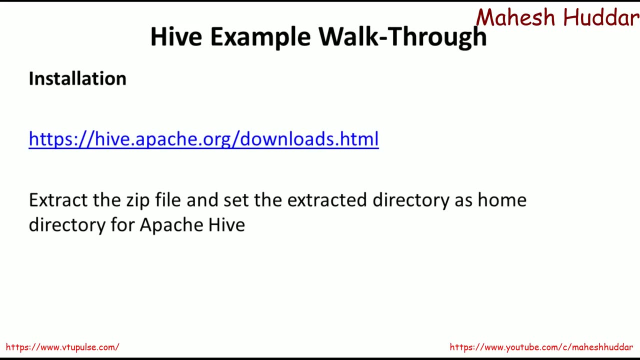 it will be given back to driver, The driver in turns given back that result to the user through the interface. So this is how the Apache Hive works. Now we will take a very simple example to understand the HiveQL queries. If you want to execute HiveQL queries, we need the Hive should be installed on our 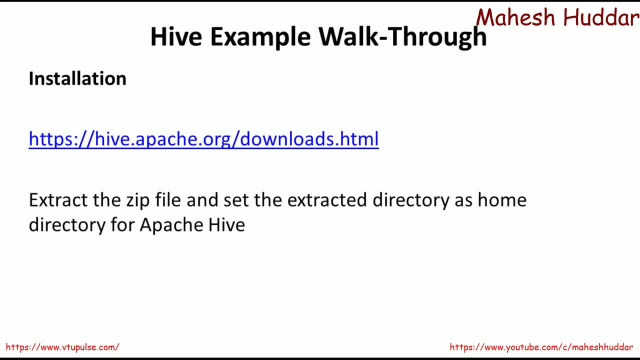 machine To install Apache Hive. first we need to go to Hive, Apacheorg to download that Apache Hive. Once the Apache Hive is downloaded, we need to extract that particular zip file and then set the extracted directory as a home directory for Apache Hive. 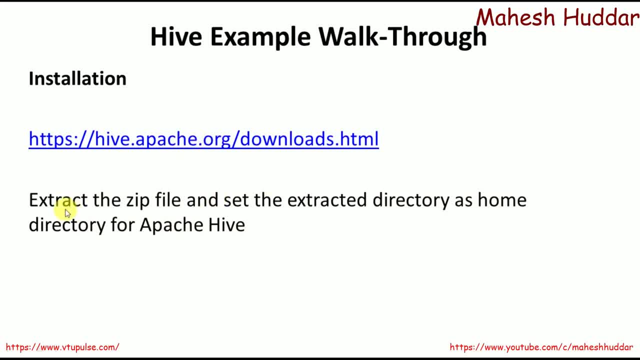 These are the three things we need to do. First we need to download it, extract that particular zip file, and then we need to set the extracted directory as a home directory. or, if you want to put it into some other directory, you can copy the content of extracted file and then set that directory as a home directory. 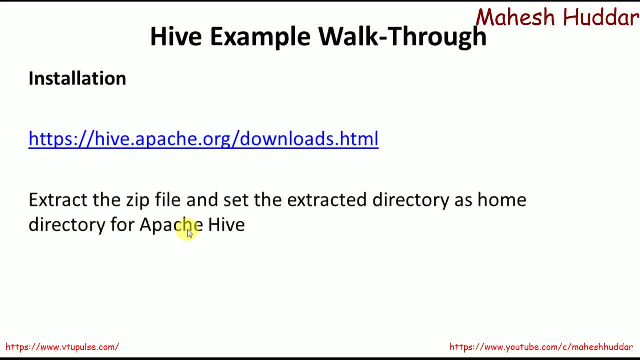 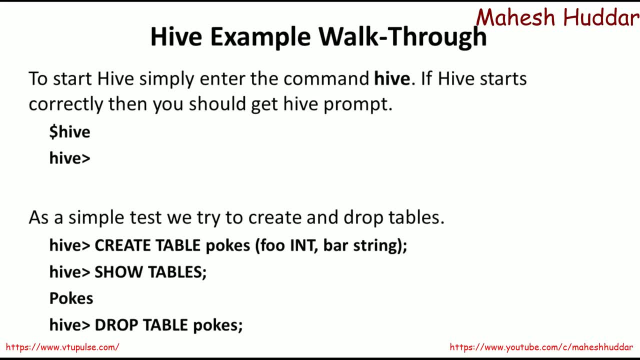 for Apache Hive. So these are the three things we need to do if you want to install Apache Hive. If you want to get the Hive prompt, we need to execute the command that is Hive. If everything is fine, then we will get a Hive prompt. 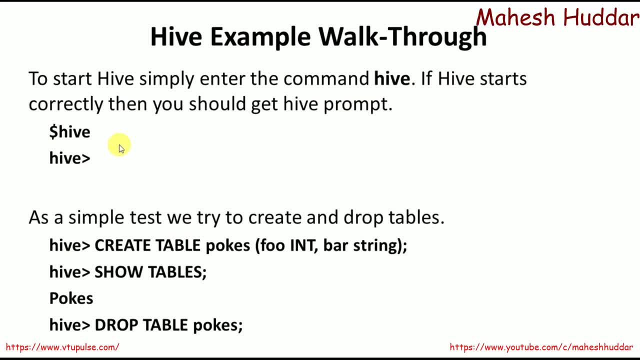 Here we can write our HiveQL queries So that we can create table. Here we can write our HiveQL queries So that we can create table, we can create a database, we can drop a database, and so on. Everything can be done. 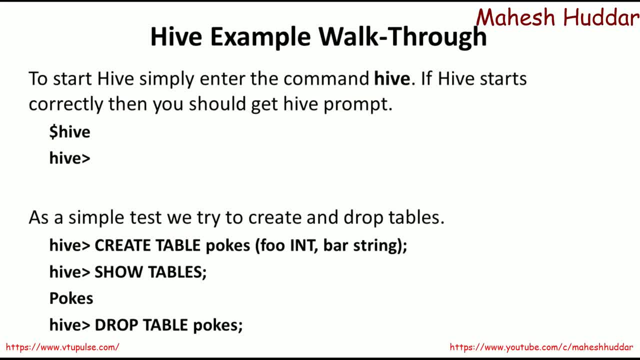 So we take a very simple example: to create and drop a table, So the create table. if you want to create table, we need to use create table query. that is, create table- the name of the table, followed by we need to pass attribute names as well. 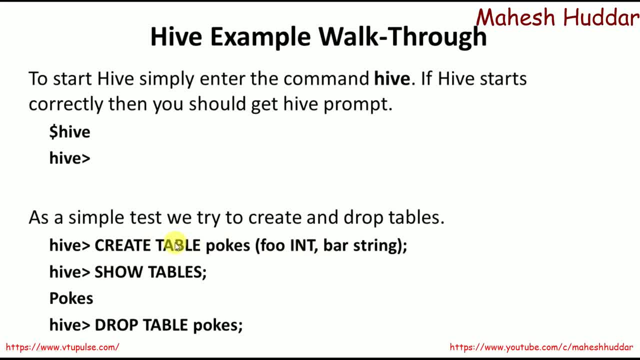 as the type of attributes as a parameter to create table. So in this case, create table pokes. the two attributes are there. One is a foo, One is of type integer. the bar is of type string in this case. So if it is executed successfully, you will get an OK message. 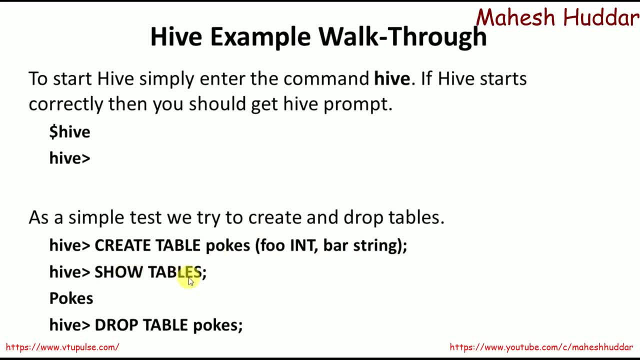 And then if you want to see the tables which are created, you can use show tables. So it will give you definitely this particular table name if it is successfully created in the previous query And if you want to delete this particular table, we can use drop table. 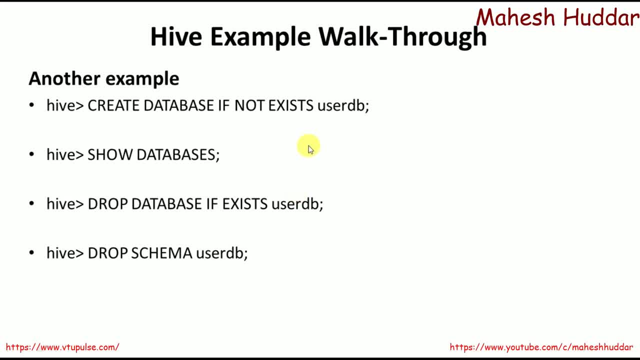 So we'll see some more HiveQL queries. If one wants to create a database, he can use create database, Create database query. and the query looks something like this: Create database if not exist. If it is already present, there is no need to create again. 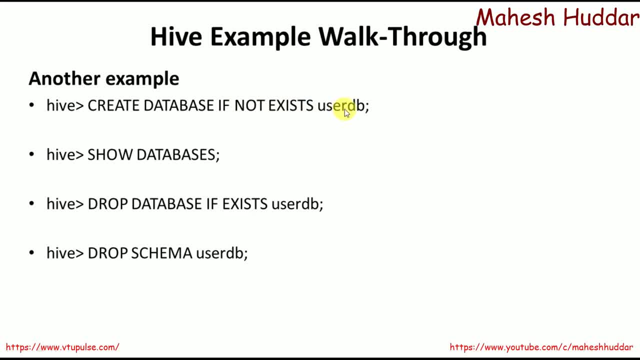 So you can use the condition like: if not exist, then create this particular database. If one wants to see the database, which is which are available in the system, he can use show databases. So it will list all the databases available in the server. 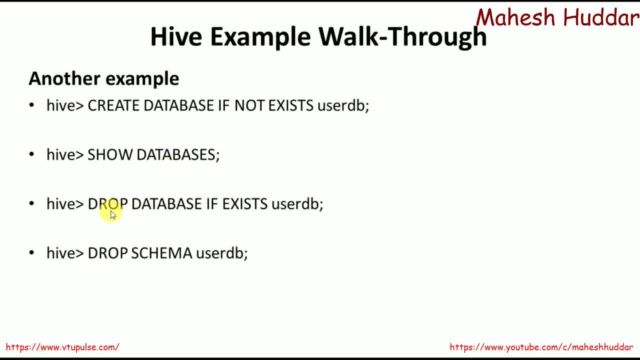 The next: if one wants to drop the table or database, he can use drop database. Next, if one wants to drop the table or database, he can use drop database And then followed by database name. And then, if one wants to drop a schema, he can use drop schema and then followed by the. 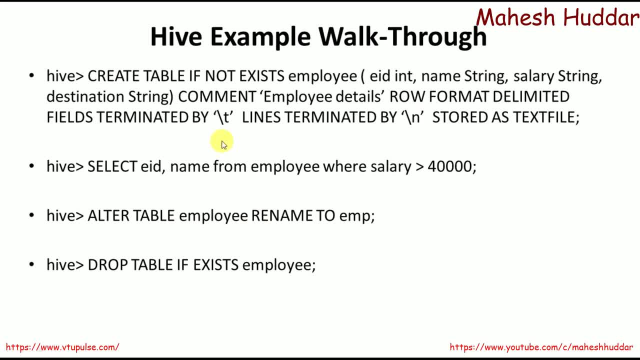 schema name. Okay, if you want to create a table, he can use create table followed by the table name. The parameter to it is the attribute name followed by the type of attribute. So that is the parameter to the create table. So, in this case, create table. employee. 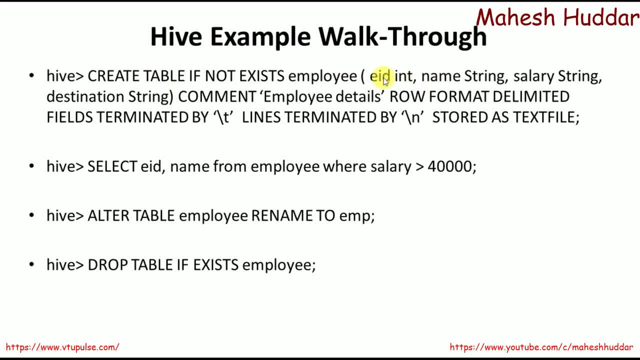 It has four attributes. The one is the employee ID, name, salary and destination, And there are some optional parameters you can use. One is called as a comment, which is used to specify what is the type of table, is this and so on. 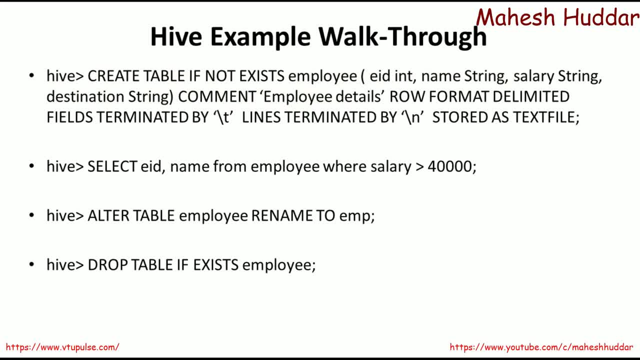 So it is just to give an information about that particular table. That's the only intention. In this case it is given as employee details. So if one sees the content of comment he can easily understand what kind of data is available in this particular table.